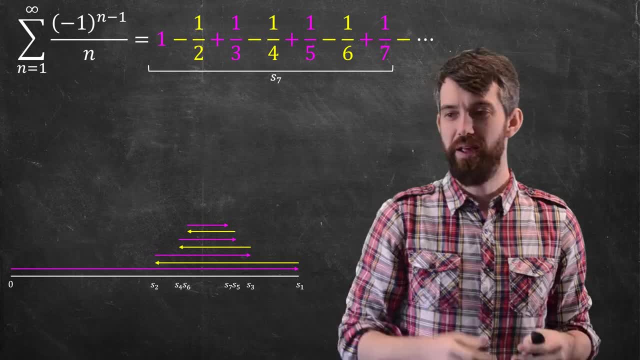 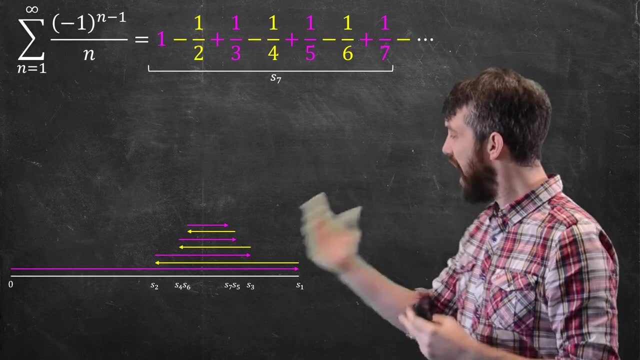 And then I advance to my s6, and advance to my s7, and so on. That is because of the nature of this alternating series. there's this sort of back-and-forth process and it kind of looks like it's going to converge. 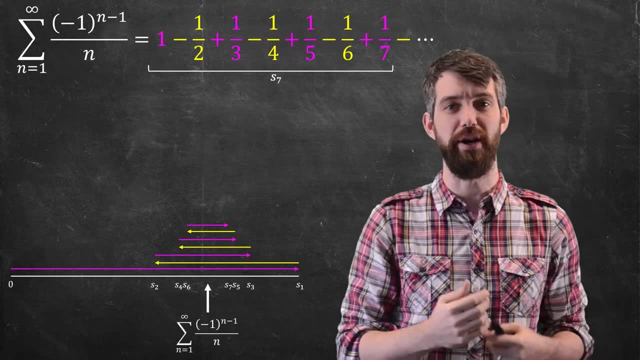 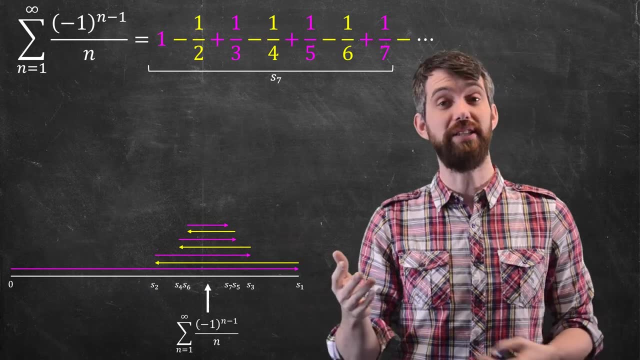 that the actual value of the series is going to be stuck somewhere here in the middle. Now, if we look at all the even partial sums- the s2, the s4, the s6, the even sums is an increasing sequence. Well, the odd partial sums- the s3, the s5, the s7,- 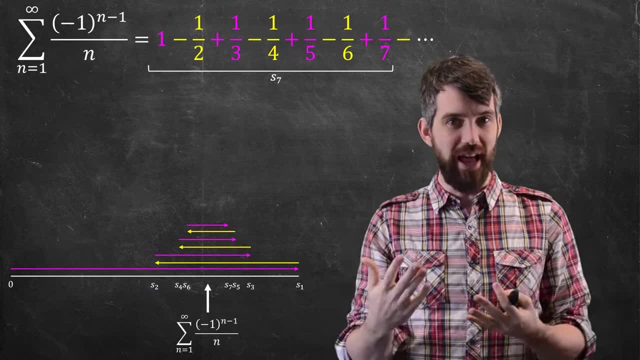 the s6, the s8, the s9, the s8, the s9, the s8, the s9, the s10, the s11, the s12, the s13, the s14, the s15, the s16, the s21, the s21, and so on. 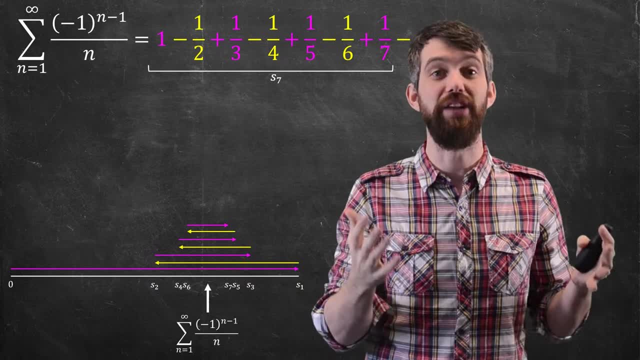 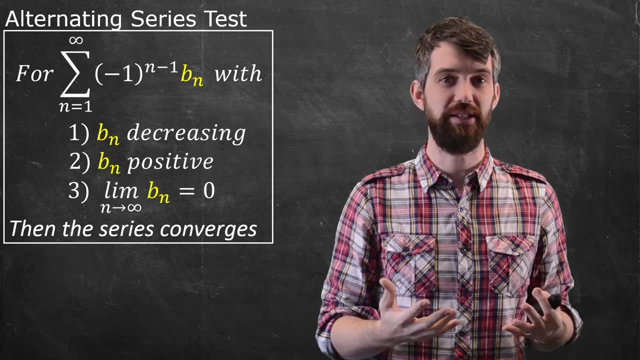 And then we start to get a decreasing one. it's getting smaller. So the final answer appears to be squished between these two different sides. Let's formalize this idea into a theorem. I'm going to say that the alternating series test says: 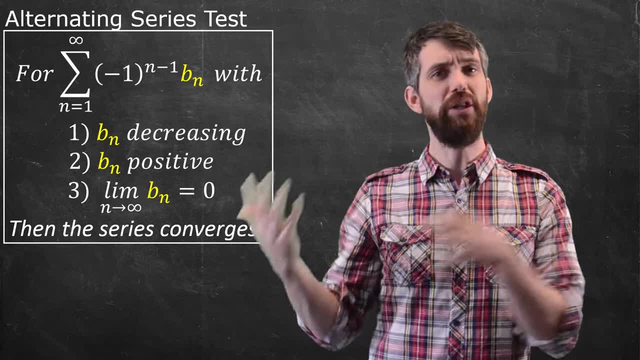 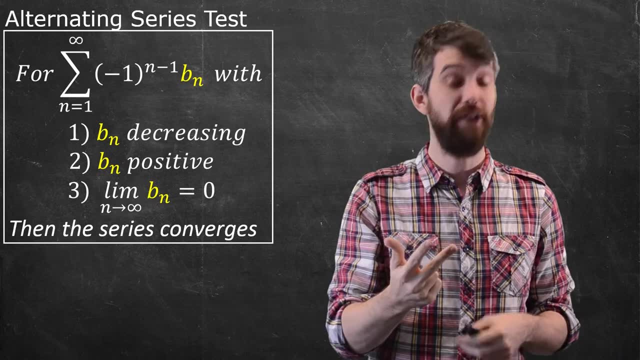 if I begin with an alternating series, so minus one to the n, minus one times a bn, some sequence that looks a lot like it did for the harmonic series, where it's going to be decreasing, where it's going to be positive. 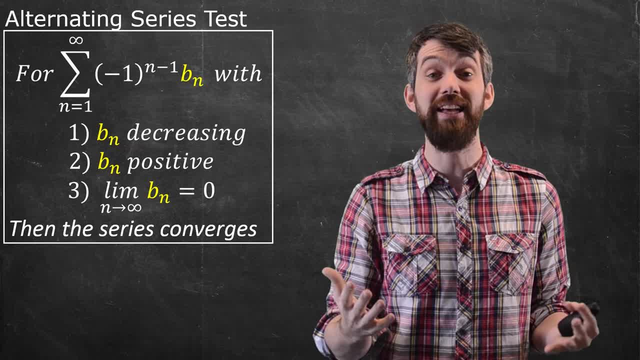 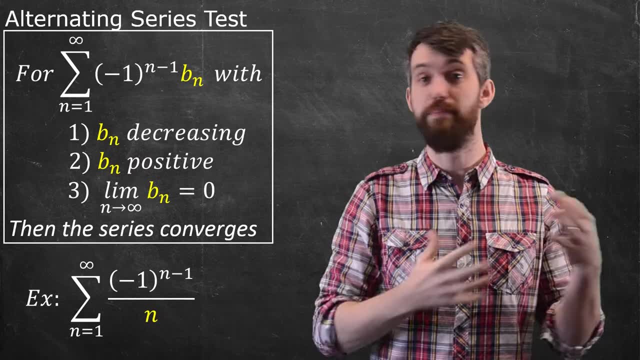 are true, then we conclude that the series converges, and that is our alternating series test. Let's see it for this specific example. So for this example, this minus 1 to the n, minus 1 divided out by n, well, what do we have? 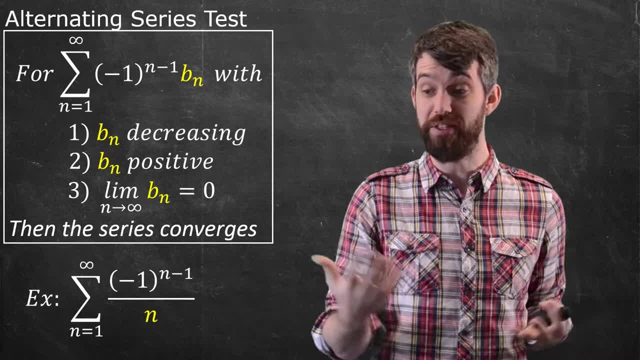 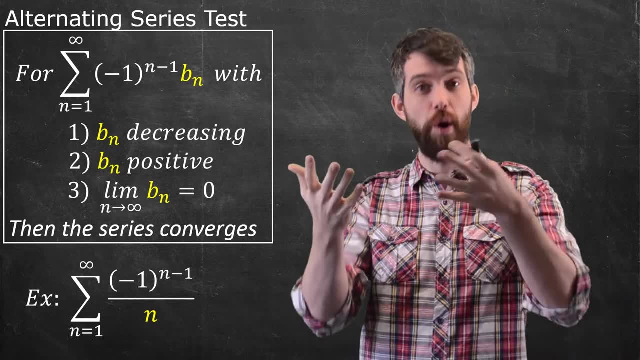 It's certainly going to be the case that the bn is positive. So the bn in this example is just 1 over n. It's positive. It's decreasing as n gets larger, 1 over n gets smaller and the limit of 1 over n is just 0. So this satisfies all three. 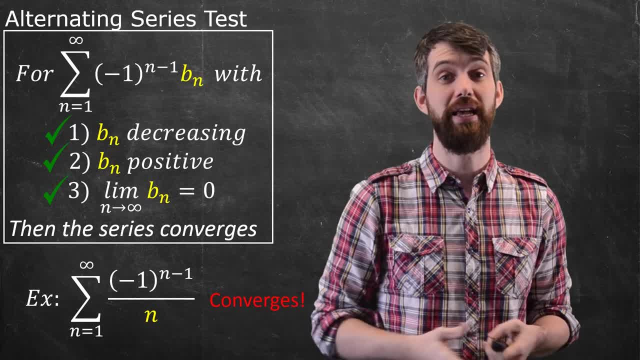 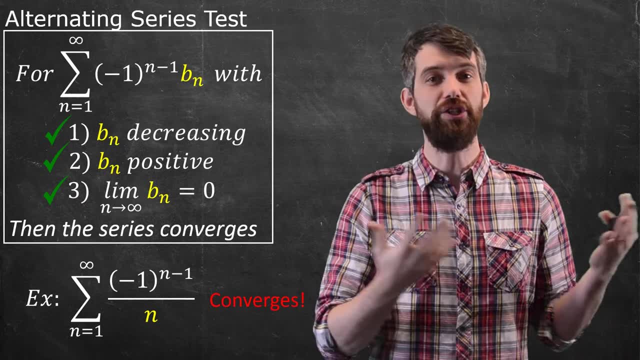 conditions of the alternating series test, and so we say that it converges. Now, alternating series are really nice, and part of the reason why they're so nice is that they're easy to check. That is this final condition: that the limit of 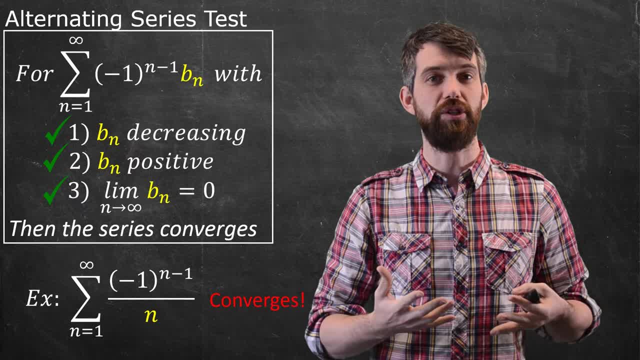 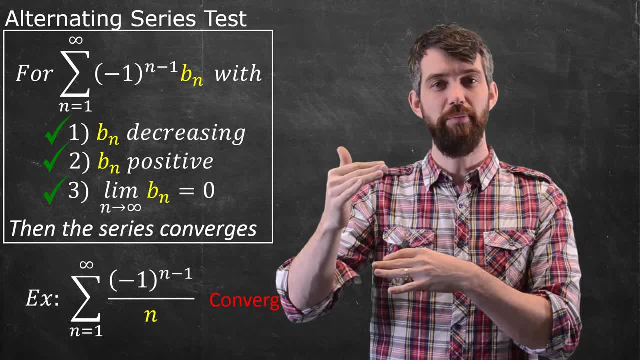 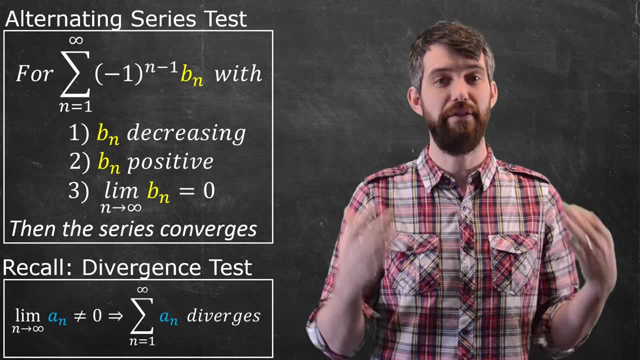 the top divided by highest power on the bottom type of analysis. But I want to contrast this with a different theorem that we've seen, which was the divergence theorem. So how did the divergence theorem work? It said, if you take the limit of the sequence and the limit of the sequence is nonzero, then the 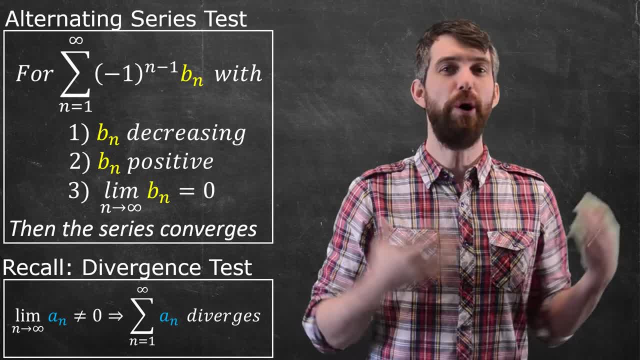 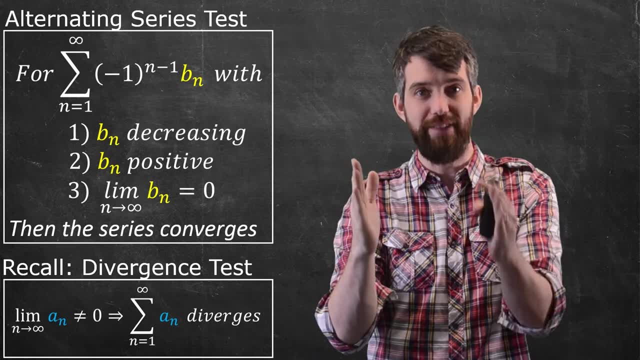 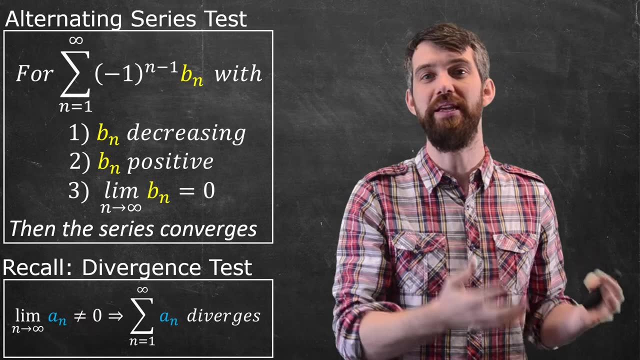 sequence diverged. and this makes sense, because suppose your limit of your sequence was- I don't know- seven, Well then the series would be getting very close to 7 plus 7 plus 7 plus 7, which would diverge. So indeed, it said, you had to have the limit being 0 if you wanted it to converge. 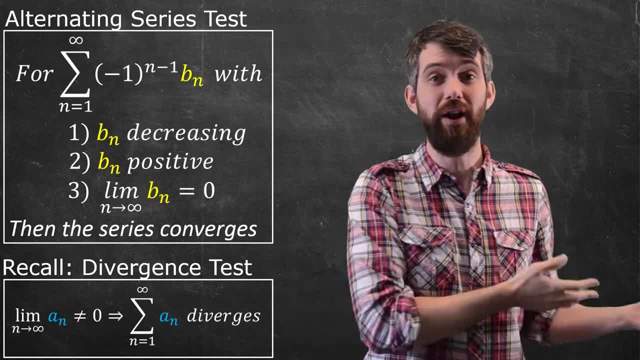 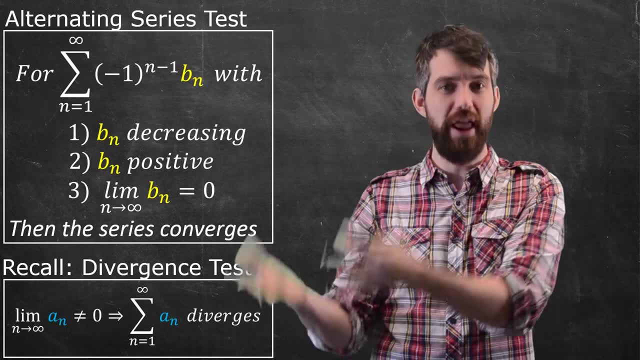 But notice that this is not an if and only if, It's not a statement with a converse that goes the other direction. Namely, it only works in the direction: if it is non-zero, then it diverges. If the limit was 0, the divergence test doesn't tell you anything at all. 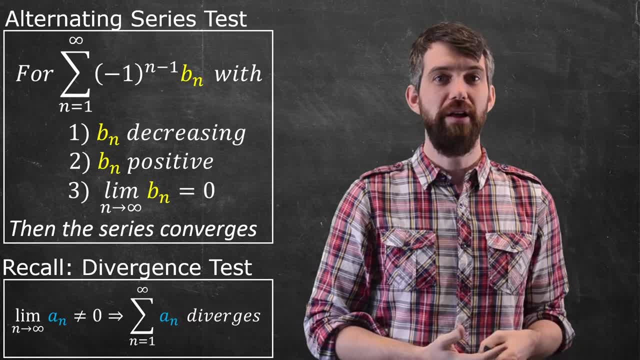 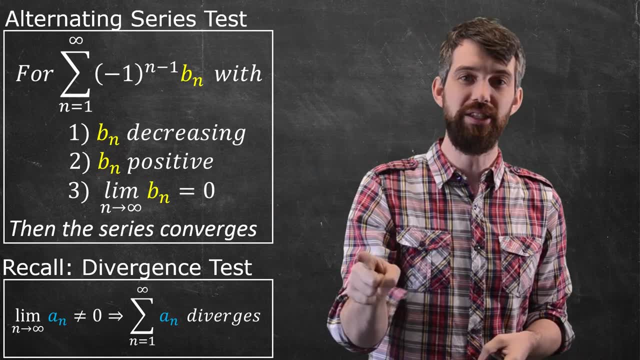 So how can I think about the alternating series test? Well, the alternating series test is like partially going the other direction of the divergence test. It says: well, if the limit is 0, and you have these other things, that needs to be alternating. 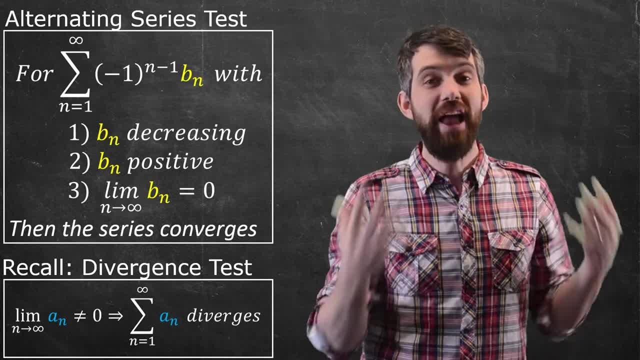 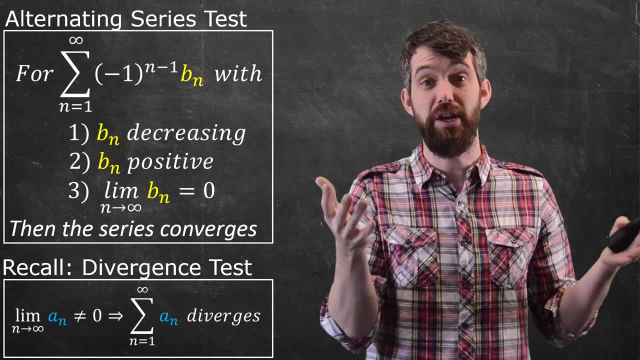 it needs to have positive terms, it needs to be decreasing, then you get convergence. So if you have the limit being 0, but you don't have any of those other things, there's no guarantee that it converges. If the limit is non-zero, then it does guarantee its divergence by 0.